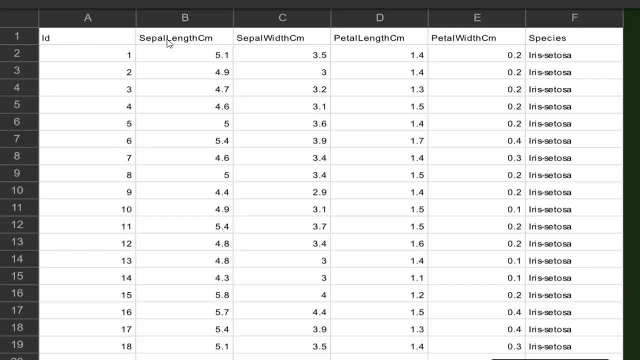 are total six columns. First one is id: sepal length, sepal width, petal length and petal width. The last column is actually the output and it is species: iris setosa. Same way, there are different species of flower and all the data is listed in a CSV file. We are going 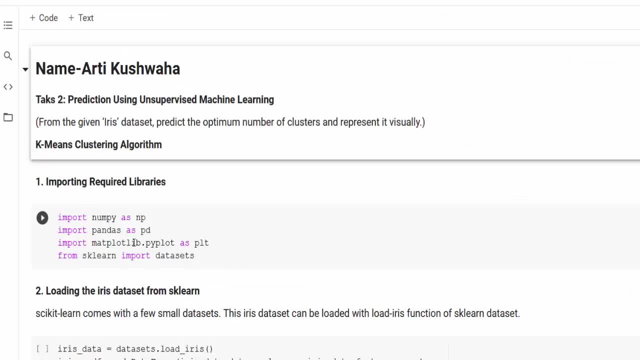 to predict optimal number of clusters. So first of all we need to import required library. We need to import these numpy, pandas, matplotlib for plotting and then sklearndatasets to download iris dataset. So first of all we will load the iris dataset from the sklearn. 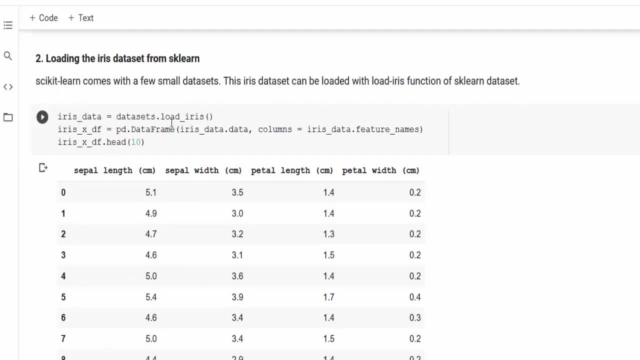 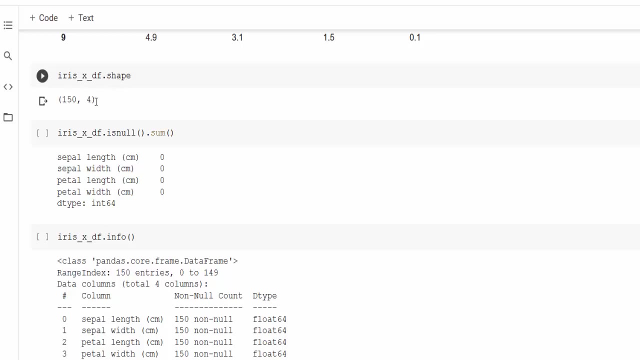 For that we need to use load iris, So datasetsloadiris will load the data. Then we can convert this iris data into panda data frame and it will show our data like this: Next, using save, we can find out the rows and columns of dataset, like 150 rows and 4 columns. 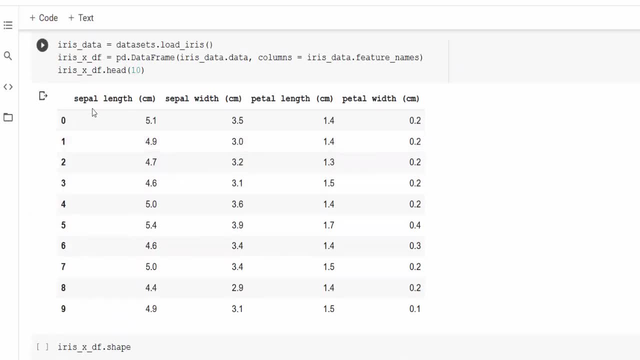 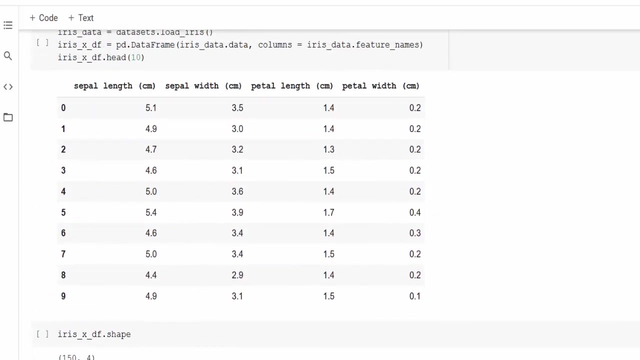 in this iris dataset. Actually, here you can see we have only 4 columns like sepal length, sepal width, petal length and petal width. It's not showing id and the output or species column, So only 4 columns here. These are actually feature columns and on these feature. 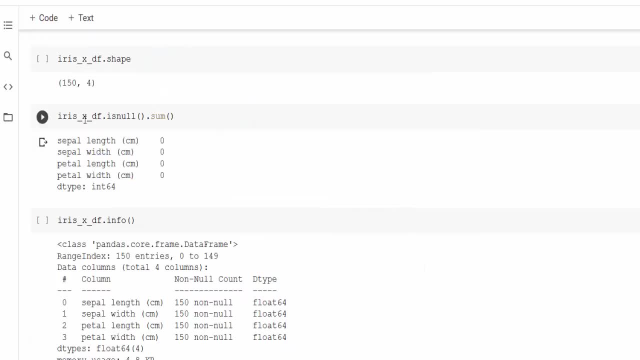 columns. we will apply the kmean clustering configuration. We will use the kmean clustering algorithm. we can also use is null dot sum function to figure out if any column is null. no column is null, as all the values are 0. then we can also use info. 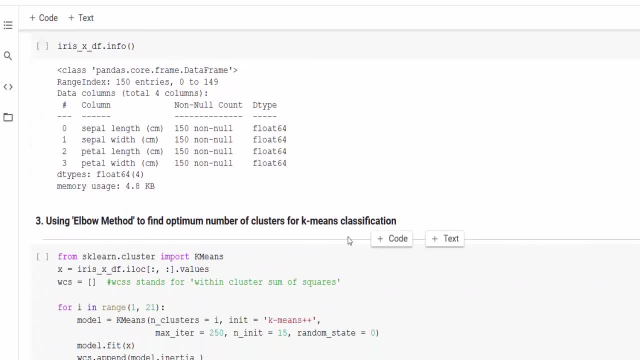 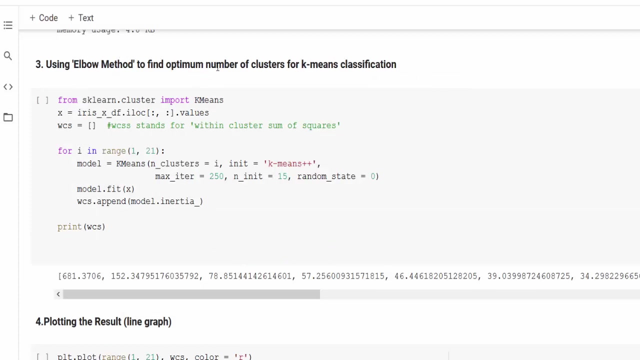 to get other information about the data frame, like: sample: length has 150 rows and no null values, and all the data types are float. 64, which is a decimal value. sable width has 150 rows and no null values, and all the decimal values. now we are going to use algo method to find optimal number of clusters for K. 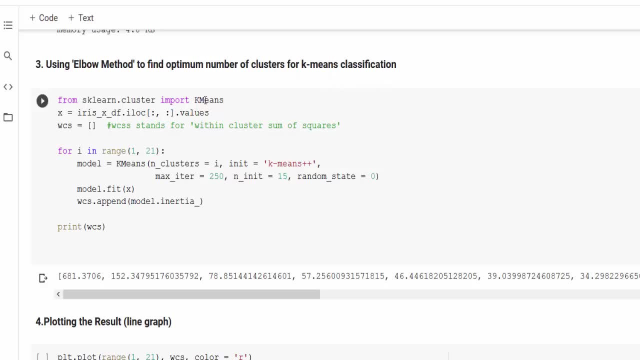 means classification. here first of all we need to import the K means model from sklearn dot cluster and then we need to find out wcs, which is within cluster sum of squares. so here we set the model k means and then we deils out which is fits the requirement. we need to set it first. 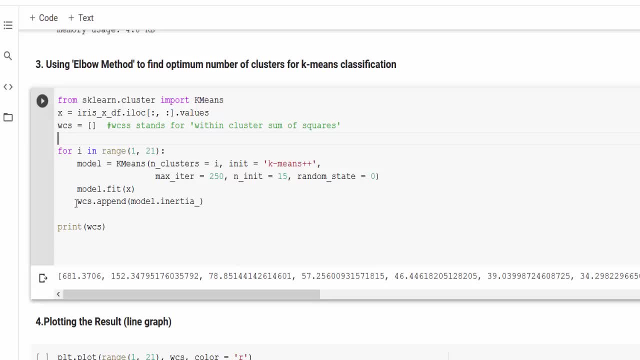 and after that we go to the next chapter, seeds. then we stay here and check, we train it using modelfit and after that using modelinertia we will append all the wcs values into wcs list and here we print the list of all the wcs values. 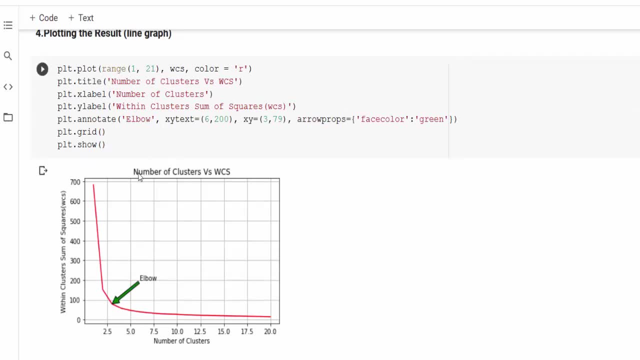 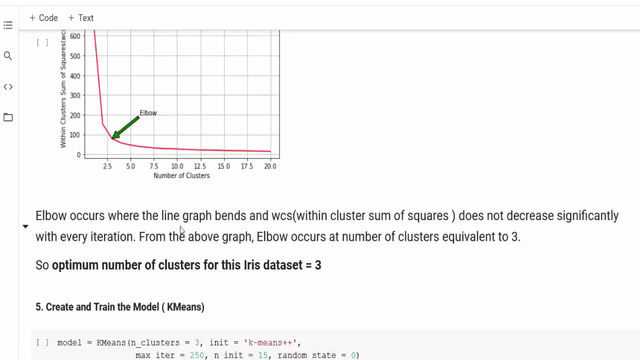 Now we are going to plot this wcs values. We are plotting number of cluster vs wcs values To find out ELBO. ELBO occurs where the line graph bends and wcl does not decrease significantly with every iteration From the above graph. ELBO occurs at the number of clusters equivalent. 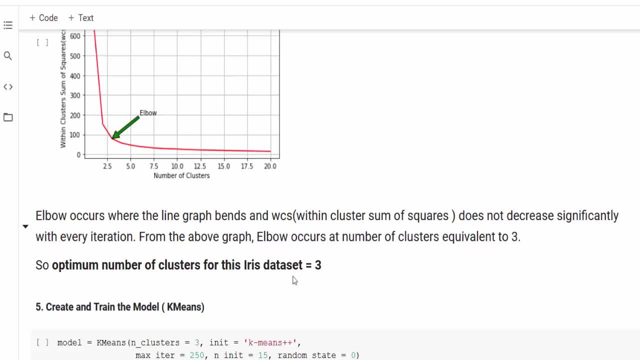 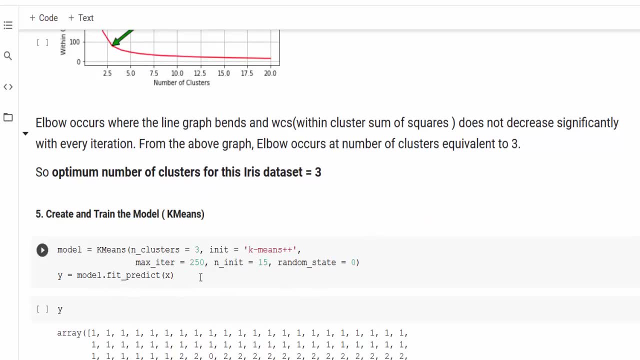 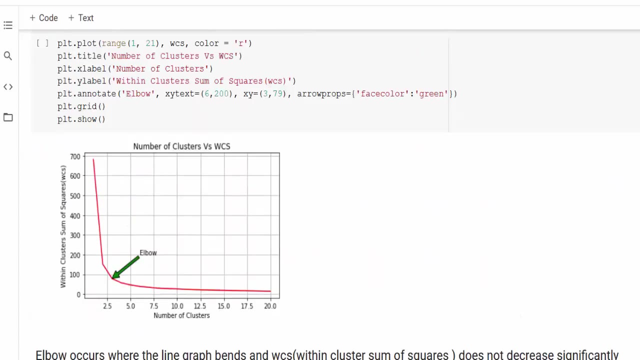 to 3.. So optimum number of cluster for this iris dataset equivalent to 3.. So again, we will set the model, we will again train the model and this time we are going to set number of clusters equal to 3.. If you remember, last time we did not set any number. 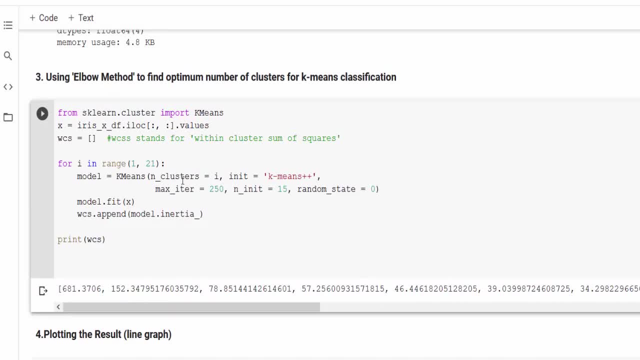 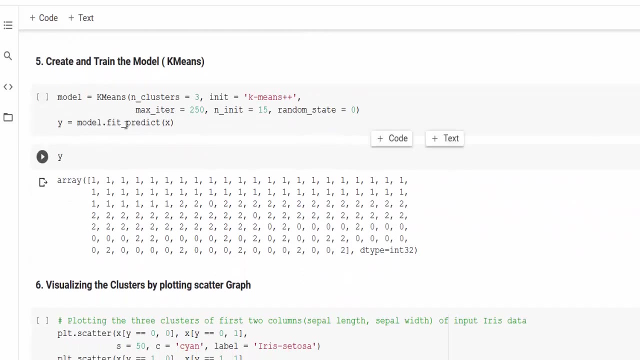 of cluster, and we just put here number of clusters equals to i. We figure out the wcs values for different values of number of clusters and then we plot it and figure out the optimum value of n is 3.. Then we are going to use this n is equal to 3 into our model. and here is the model we 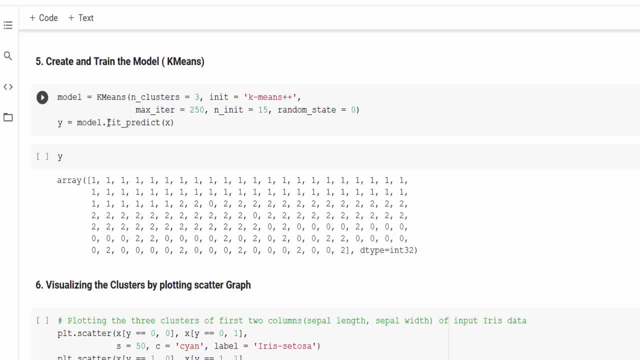 fit predict is used to train and also predict the model. both functions in single function, So y is the output. This is our output array. Now we are going to plot this out here. The are going to plot this output, so for that we are going to use scatter graph. 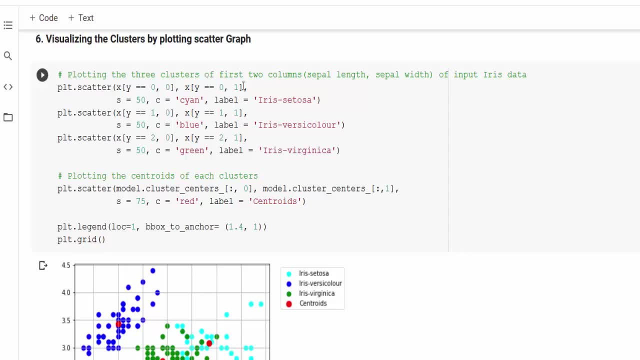 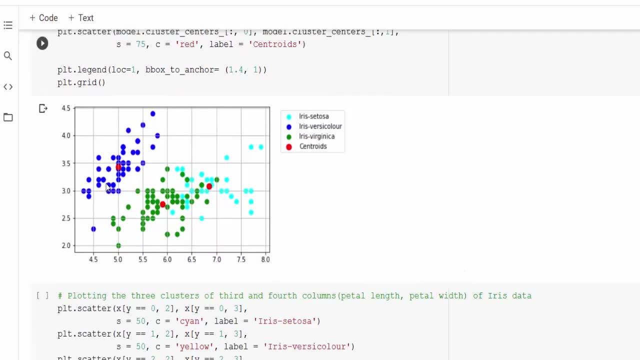 we are going to plot the three clusters of first two columns. first two columns are sepal length and sepal width. so for sepal length and sepal width here are three clusters, and three clusters are represented here using three colors, like blue, green and cyan, and centroid of clusters are represent by the red color. 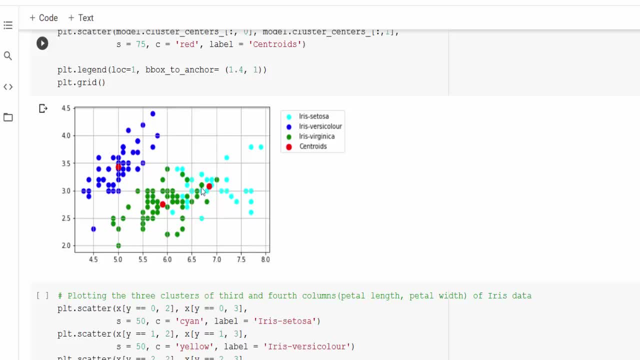 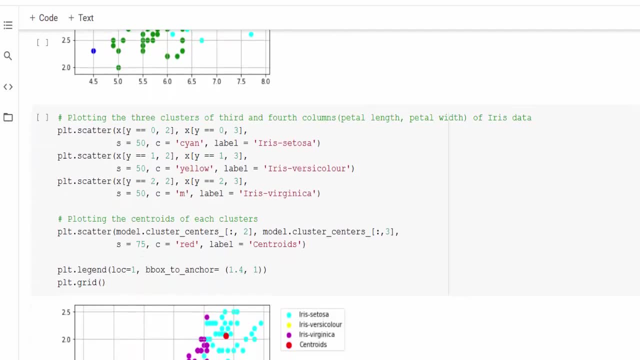 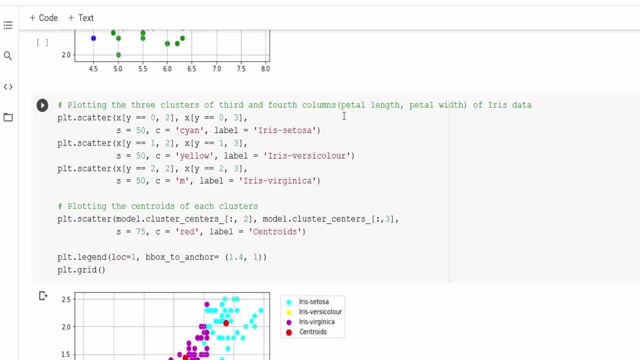 here. this centroid is of this cyan cluster, this centroid is of green cluster and this centroid is of this blue cluster. next is we are going to plot these three cluster for third and fourth columns also, that is, petal length and petal width cluster. all the three clusters are represent by different.